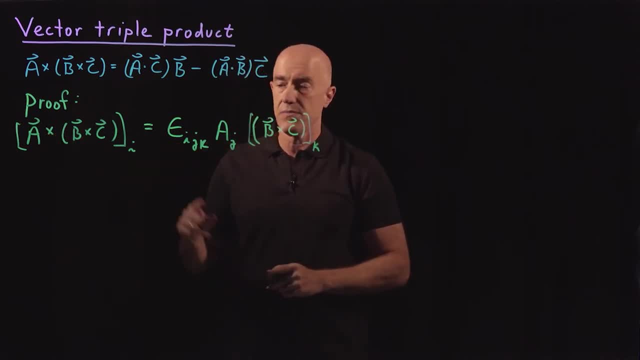 here using the Levi-Savita symbol, And then this second cross product we can write again using the Levi-Savita symbol. So we have our epsilon i, j, k, a, j, And then the k-th component of b cross c will be epsilon k. 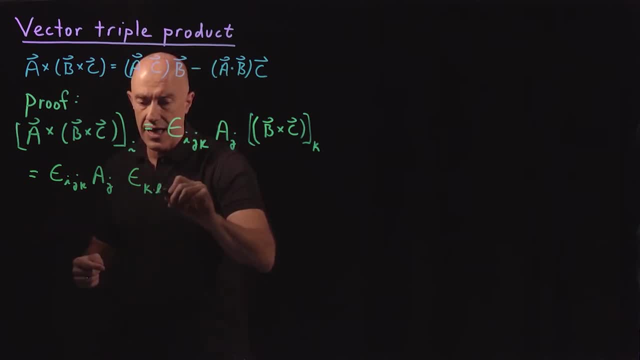 And then I'll use l m, say, And we'll have a b sub l and a c sub m. OK, The next manipulation I need to do is to put these Levi-Savita symbols together as a product. Here we're summing. 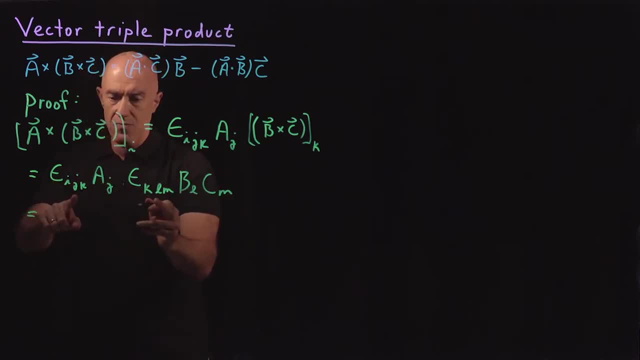 over k. I'm going to put k on one of the indices of the Levi-Savita symbol, So I'm going to want to put k as the first index. So I can write this as epsilon k, i, j using the cyclical 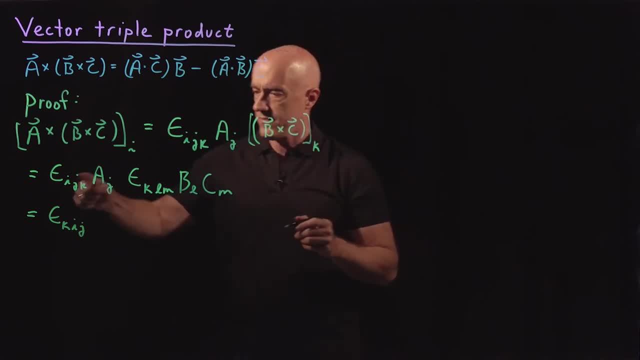 property of the Levi-Savita symbol, And then epsilon k, l, m of the second one, And then we have an a, j, b, l, c. It's 1,, 2, 3, 4, 5.. I'm sorry. 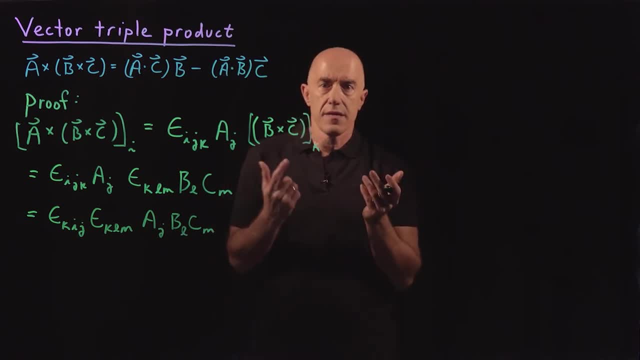 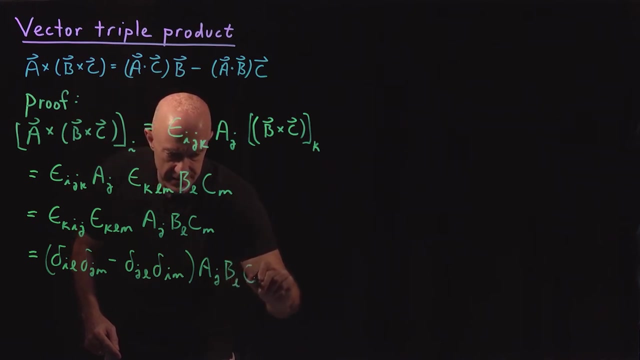 Now we use the identity that if we're summing over one index of a product of Levi-Savita symbols, then we can write that as the product of Kronecker deltas. So the product here would be delta, iL, delta jM minus delta, jL, delta iM times aJ, bL, cM. 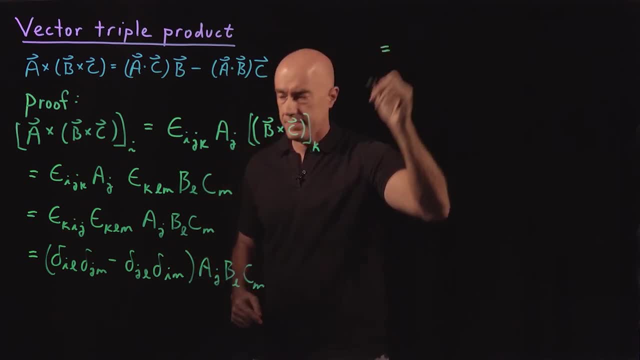 Okay, I'll continue up here. What do we do next? Well, we're going to: we have a delta iL, and that can contract the bL, and we have a delta jM and that can contract the cM. 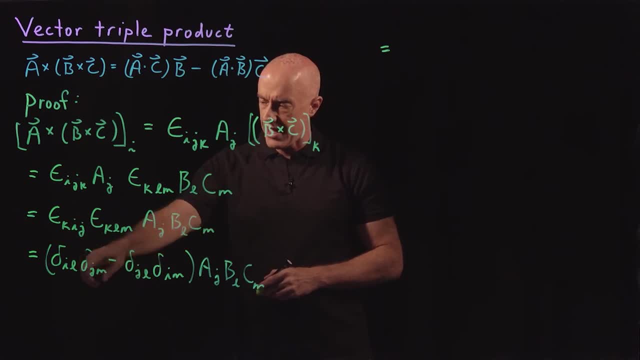 So I'm going to try and keep the i and j and then contract the L and M. So if we do the first one, delta iL times bL is bI, so we'll get aJ bI and delta jM. 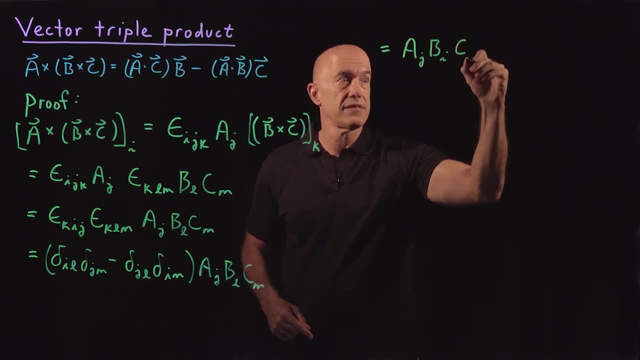 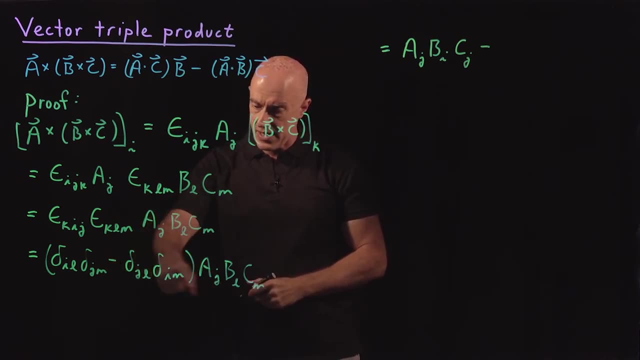 cM is cJ, so we have a cJ and then minus. now I'm going to contract the L, so we have aJ again, And then we'll have delta jL- bL will be bJ and delta iM- cM will be cI. okay, 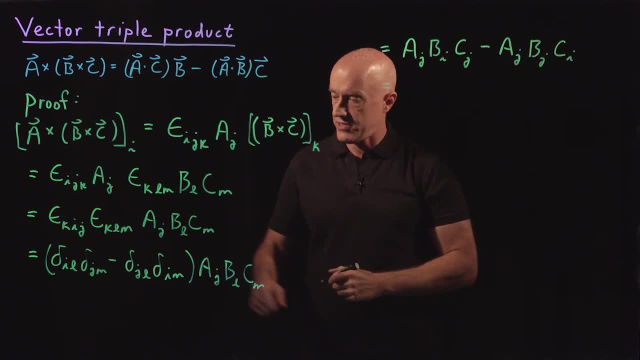 So we've used the Einstein summation convention and we contracted the Kronecker delta times one of these components of the vectors. okay, Okay, So now we don't have any Levi-Savita symbols, we don't have any Kronecker deltas, we want. 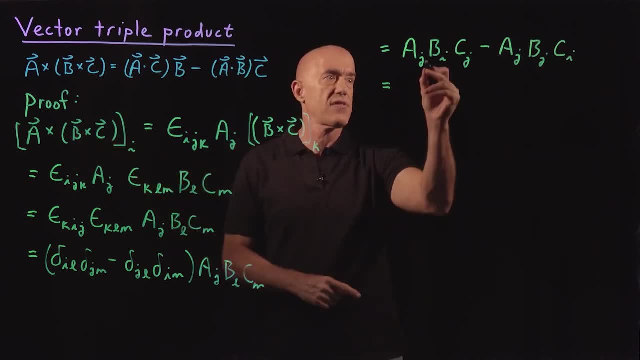 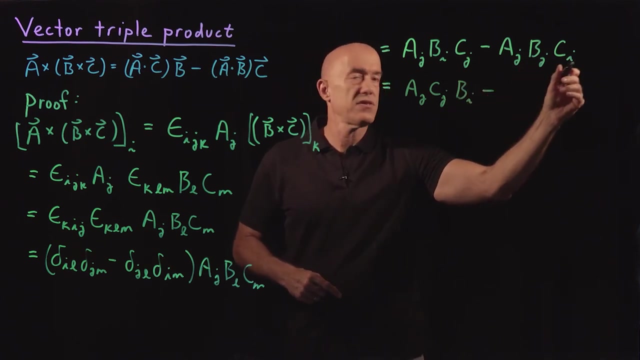 to make sense out of this. So remember we're looking at the i-th component, so i is the only index which is not summed over, so I can rewrite this: this is aJ cJ times bI, right, And this one is aJ bJ times cI. 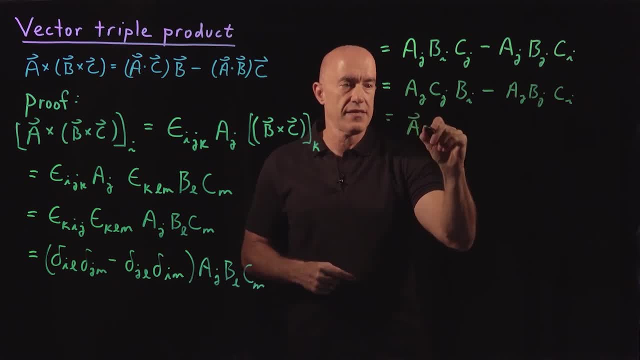 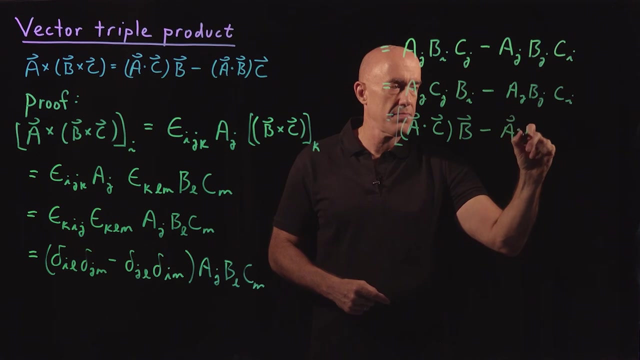 aJ, cJ is just ac, and then bI is the i-th component of the vector b, minus aJ. bJ is ab and cI is the i-th component of the vector c. okay, So we're basically done. 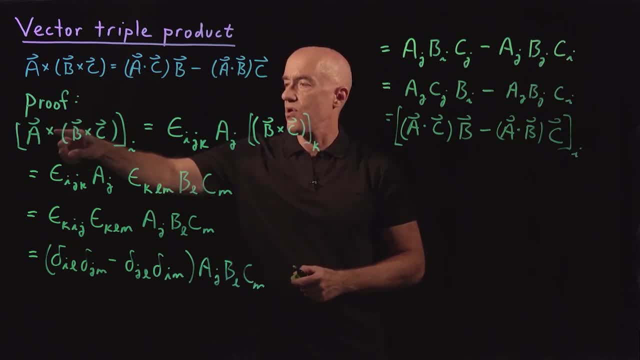 We've proved that the i-th component, The i-th component, of a cross b, cross c, is equal to the i-th component of a dot c times b minus a dot b times c. So if that's true- for i equals one, two and three- then we. what we've proved, then, is: